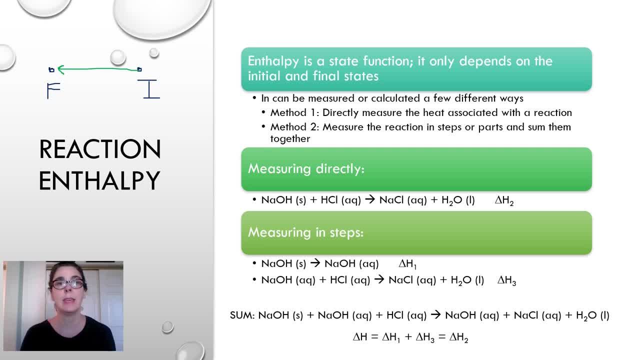 measure reactions one and three and we combine them together to give us reaction two. So it's like we're measuring the reaction in steps and if we take those steps and we add them together we get the overall reaction. So for the second part of the lab where we're kind of measuring it in steps, it's more like going 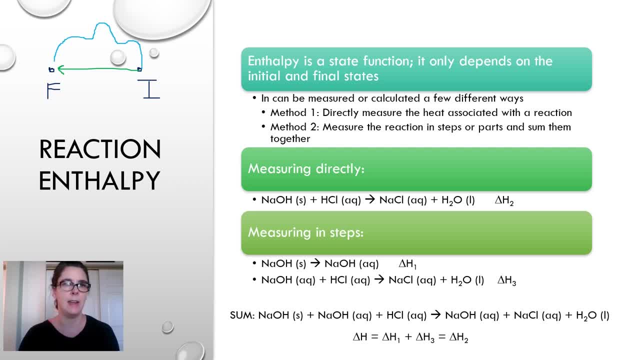 initial, and then over here and then back around and down to the final. We still get there. it just took us a little bit longer, a little bit sort of different route to get there. Okay, so let's take a look at what we're measuring today. So reaction two is the direct reaction, and that's the reaction. 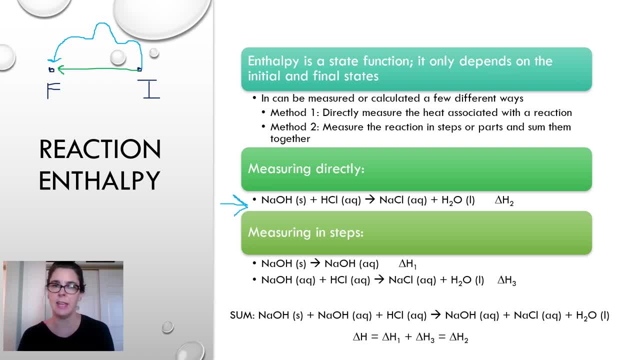 of dissolving solid sodium hydroxide into hydrochloric acid to give us sodium chloride and water. So we're going to measure the heat associated with this process for some given quantities of sodium hydroxide and water and calculate the enthalpy And then, in sort of another part of the lab, we are measuring 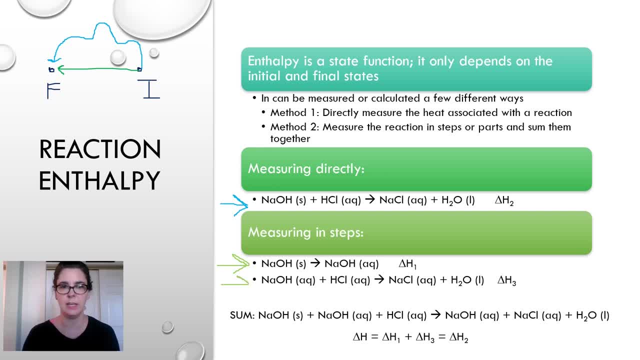 reaction one and reaction three. So reaction one is sodium hydroxide and water. So we're going to measure the enthalpy associated with that. and then, finally, reaction three is aqueous sodium hydroxide plus aqueous hydrochloric acid to give us NaCl and H2O. So if we take reactions one and three, 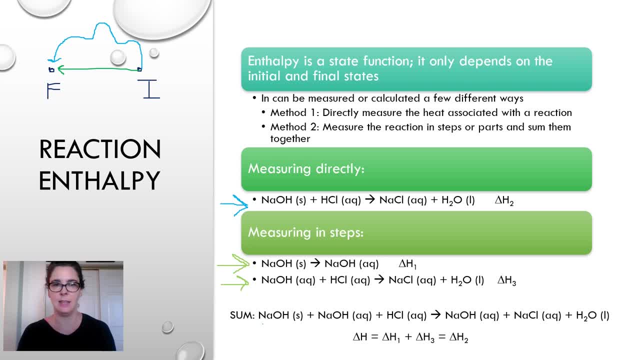 and we add them together, we get one, two, three products that come from NaOH solid, NaOH aqueous, HCl aqueous, and we get one, two, three products that we get from NaOH aqueous, NaCl aqueous and H2O liquid. Okay, so what happens then is, once we sum them together, anything that is the. 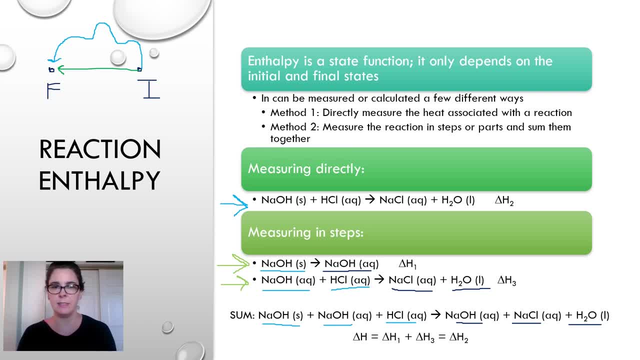 same on either side. we call those intermediates. we can eliminate So aqueous NaOH cancels with aqueous NaOH on each side and we're left with the sum of these two reactions being our direct measurement of reaction number two. So according to Hess's law, then if we take the enthalpies of 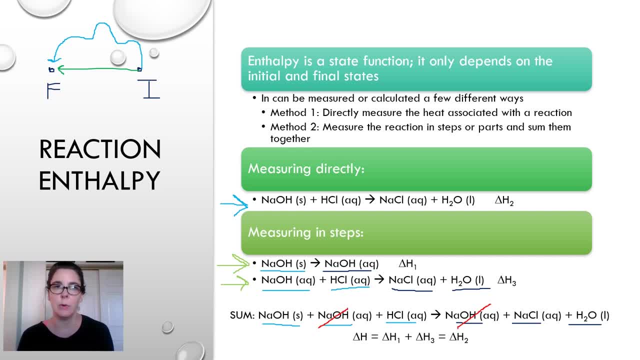 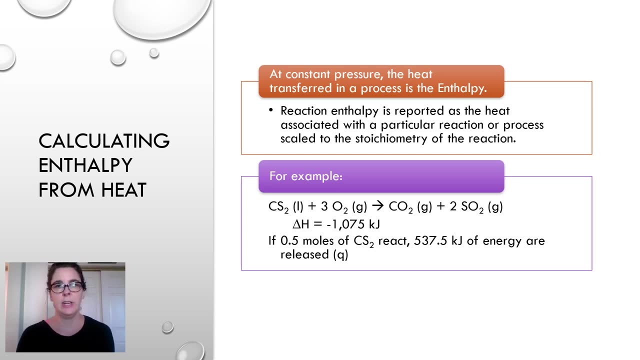 reactions one and three and add them together, it's going to be the same as reaction number two. So hopefully you'll see that in lab It should be pretty close. Okay, so calculating the enthalpy from heat. So at constant pressure, the heat transferred in a process is called the enthalpy. So we're 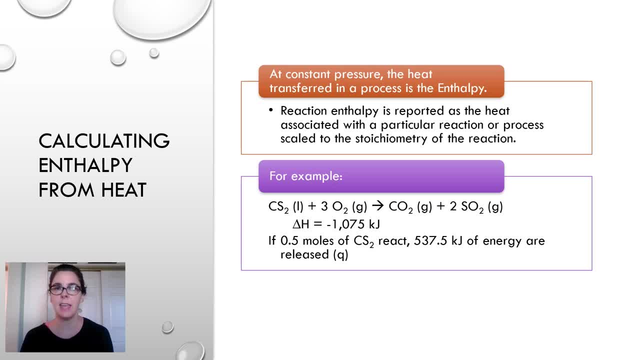 looking at reaction enthalpy, so delta H of reaction. So reaction enthalpy is the heat associated with a particular reaction, but it is scaled to the stoichiometry of that reaction. So when we're calculating or reporting the enthalpy of a reaction, we do have to change it into. 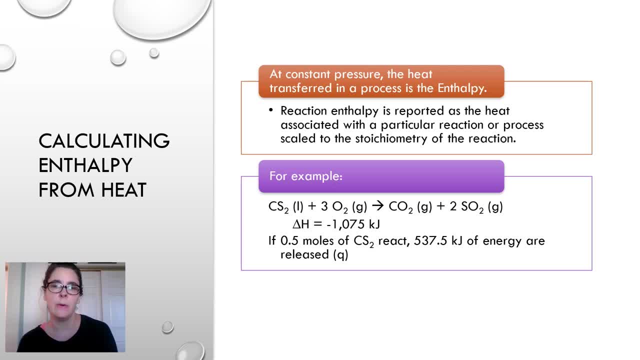 again to match the coefficients of our reaction. So, for example, let's take a look at a reaction where we have carbon disulfide reacting with oxygen to give us carbon dioxide and sulfur dioxide. So for this particular reaction the enthalpy is negative: 1,075 kilojoules. So we have an exothermic reaction that produces 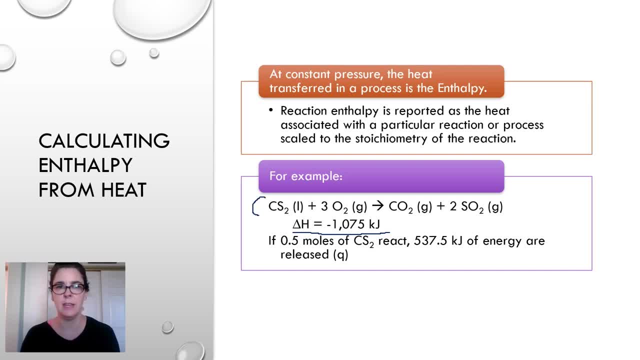 1,075 kilojoules for every one. this is a one here, one mole of carbon disulfide. Okay, so that's the enthalpy of that reaction. So if we wanted to look at different quantities then it kind of becomes the heat. So let's say, for example, we had only a half a mole. 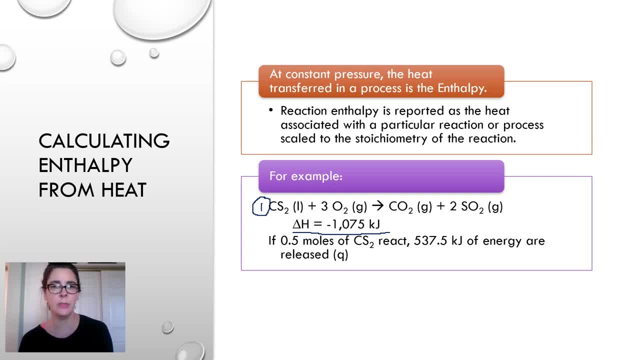 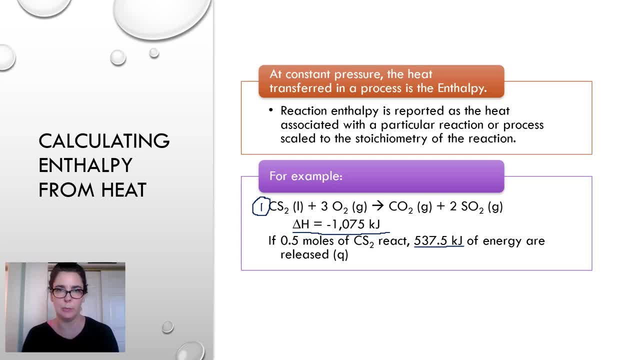 So that would be Q for that process, for that half of a mole of carbon disulfide That would be reacting in that particular process. Okay, so now let's look at Hess's law. So we're going to use that same reaction. 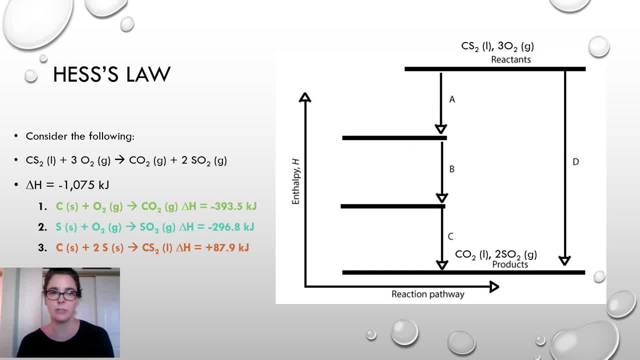 but now we're going to look at- instead of say measuring it directly, which we kind of just saw in the last slide- maybe looking now at measuring it in individual steps. Okay, so let's look at our reaction. On the reactant side, we have our carbon disulfide and our three moles of oxygen gas. 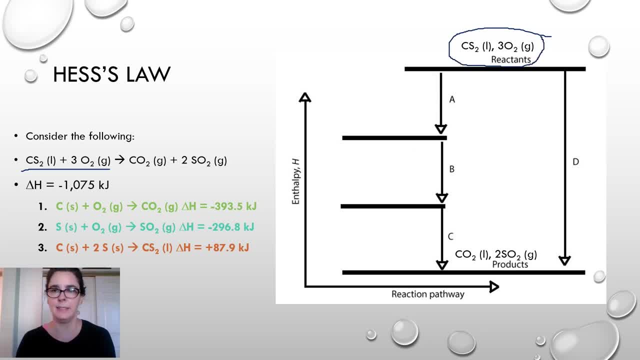 So that's right here. So the direct method is D, where we then get our CO2 and SO2, our products there. Okay, but let's think about this in terms of steps. Okay, so we could take that carbon disulfide and let's say we took that and broke it apart into elements. 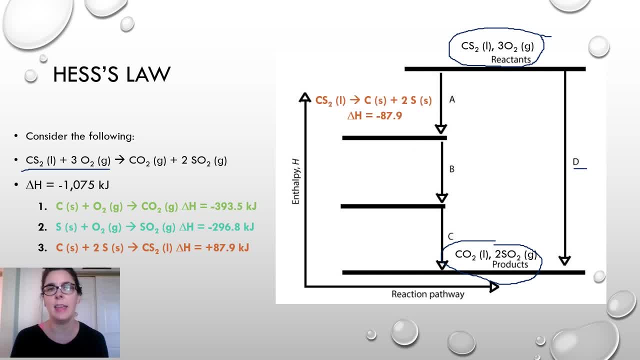 And that's going to correspond to reaction A. So carbon disulfide plus carbon to yield carbon solid plus plant greenhouse gas, which is 1.5 kilojoules, and we're going to get 1.5 CO2 per liter of carbon disulfide. So 2.5 kilometers per 크ł. Okay, so we could take that carbon disulfide and let's say we took that carbon disulfide plus 1.5 kilograms of oxygen gas, which is 1.5 kilometers per kilogram of oxygen gas, which is 1.5 kilograms per kilogram of oxygen gas, which is 1.5 kilograms of oxygen gas. 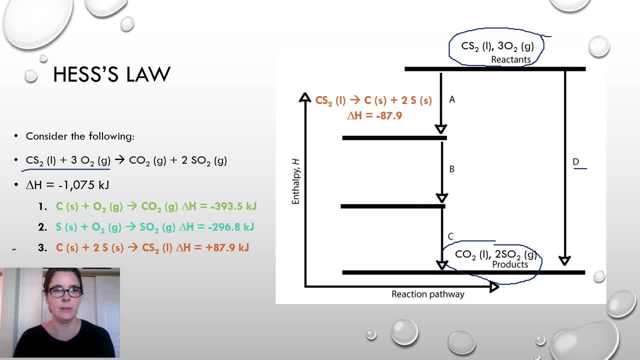 to sulfurs. okay, so that is reaction three right here. so in order to utilize this, i had to reverse that. so notice that my 87.9 kilojoules turned into negative 87.9. okay, so again, i wanted my carbon disulfide to match up with the carbon disulfide in my original reaction, so i did have to reverse that. 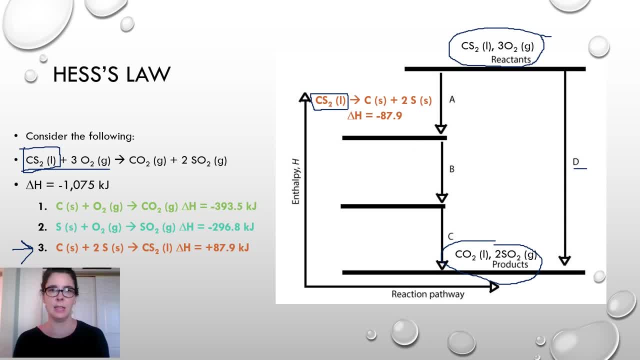 so again, that's the energy that would be associated with breaking essentially up the carbon on the sulfur into elements. okay, so then, b and c, now that we kind of have broken things up, we have carbon element and sulfur and we have our oxygen that we started with. 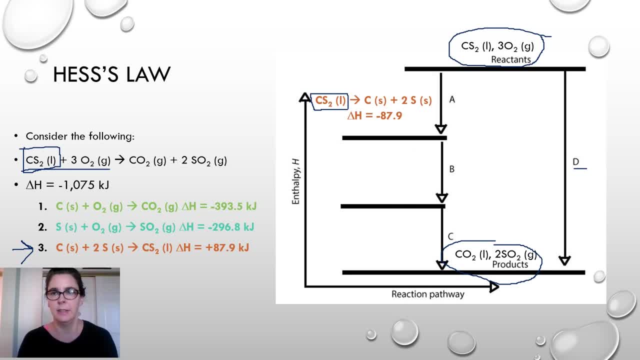 we can now start combining things together to make products. so let's take a look. so step b could be, for example, the carbon produced in step a, combining with one of our moles of oxygen gas. that was an original reaction to yield carbon dioxide and the energy or the enthalpy associated. that is negative 393.5. okay. 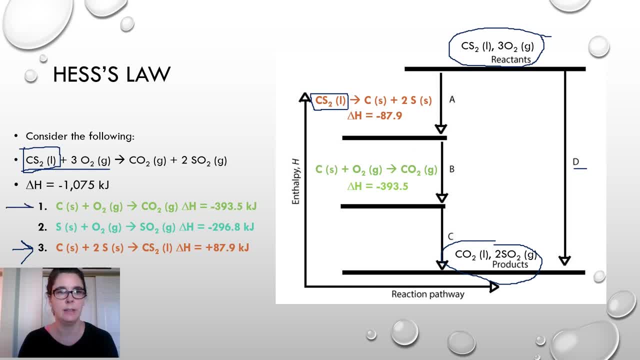 and that is given as reaction 1 up here. okay, so using reaction 1, we produced our co2 gas, which matches the co2 gas from our overall sort of desired reaction. okay, then our last step is combining the sulfur, the two sulfurs we produced in Part A, with the remaining two moles of oxygen. 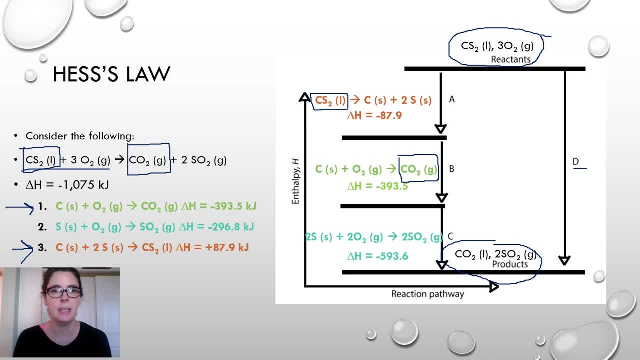 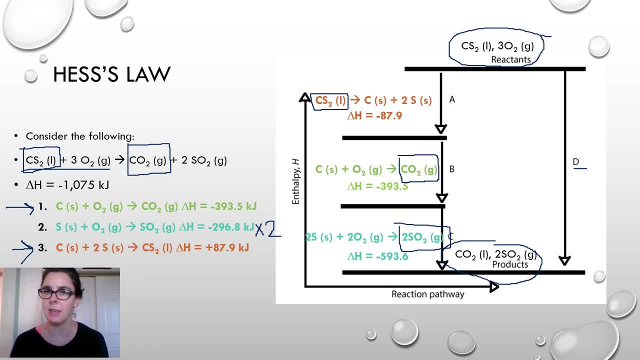 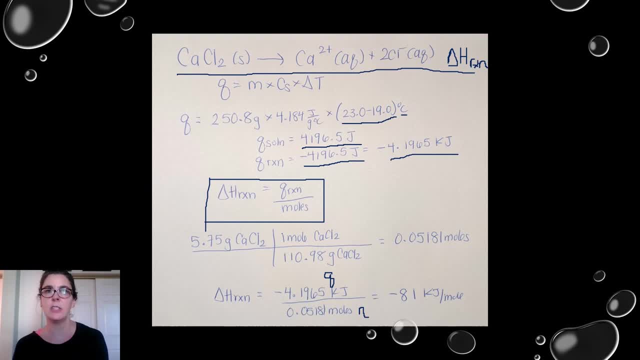 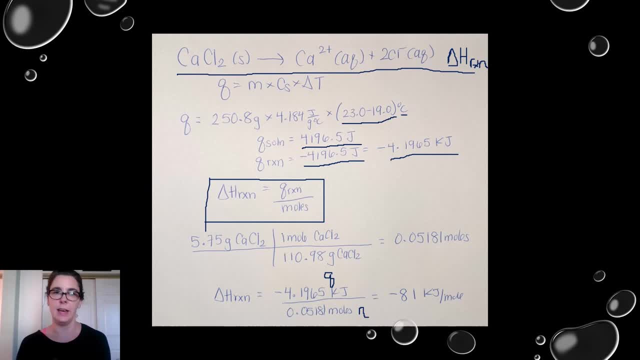 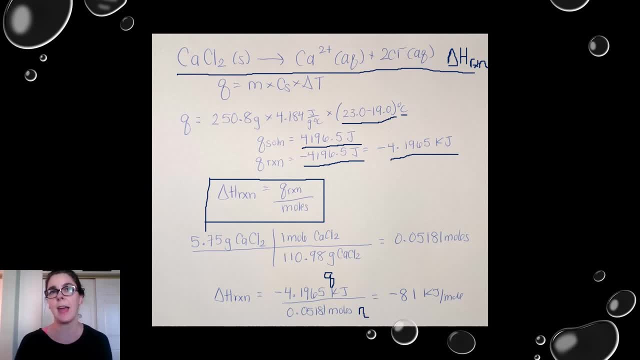 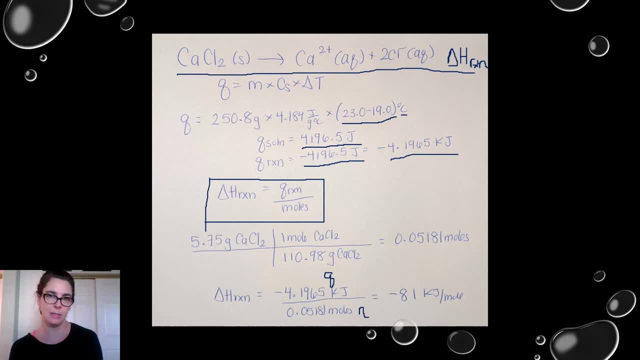 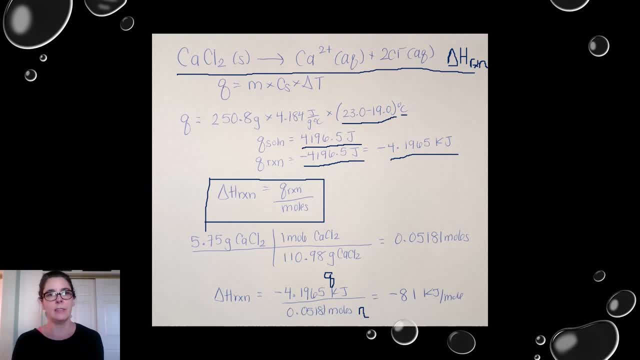 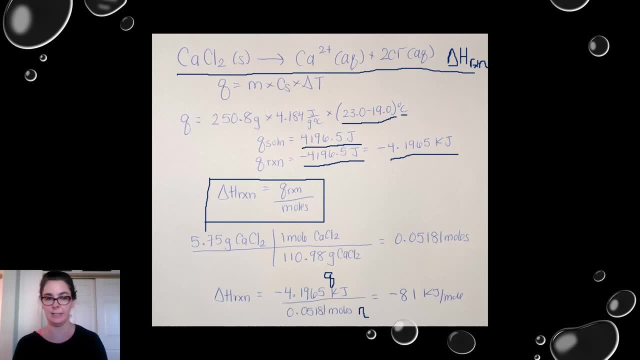 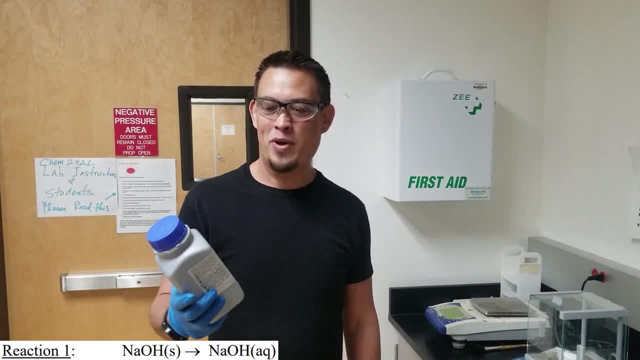 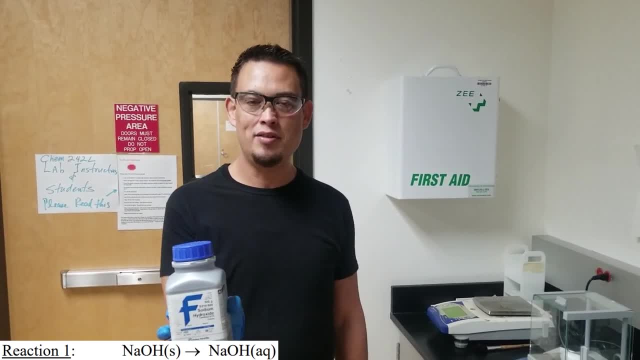 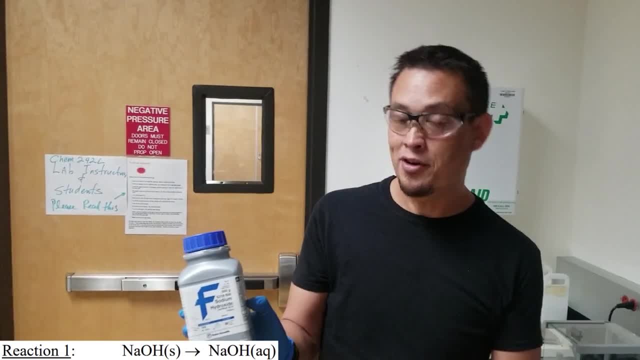 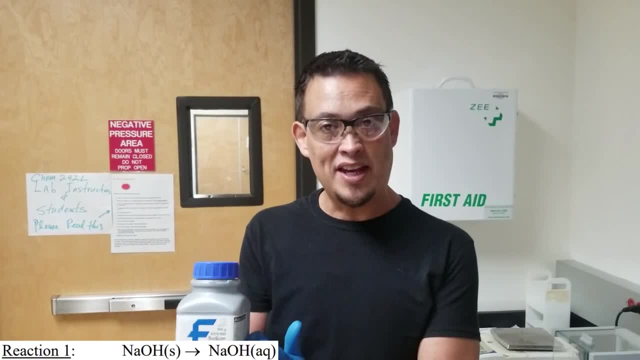 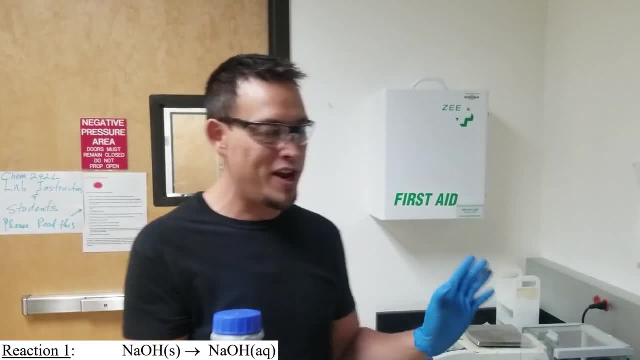 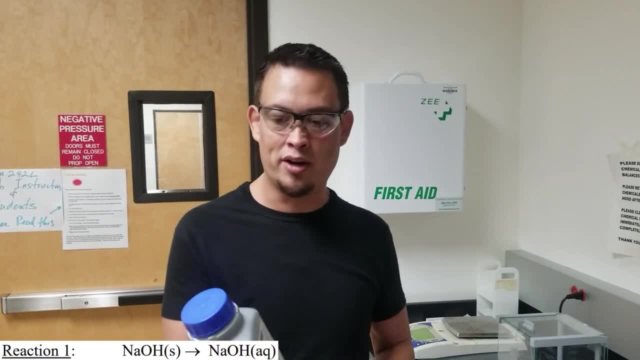 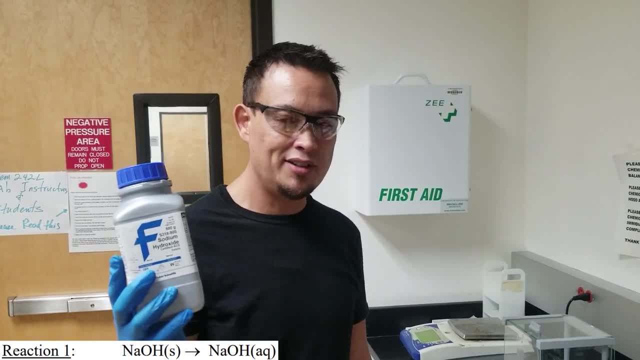 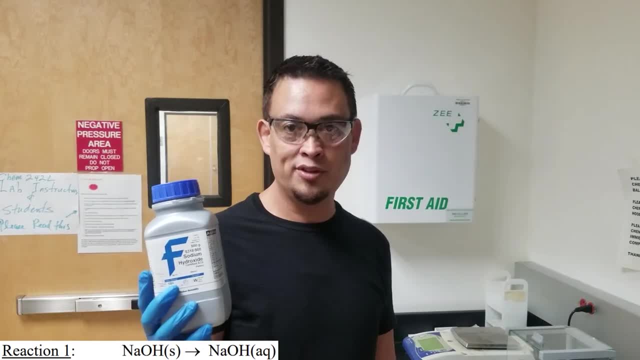 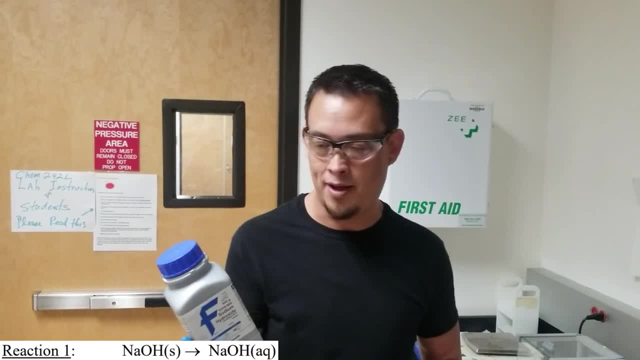 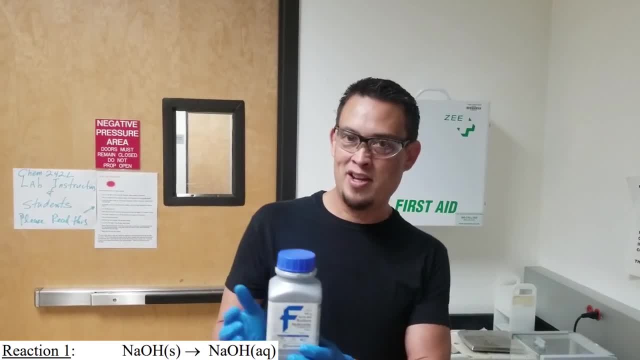 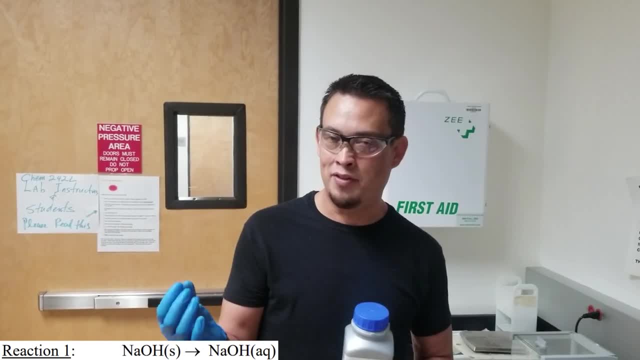 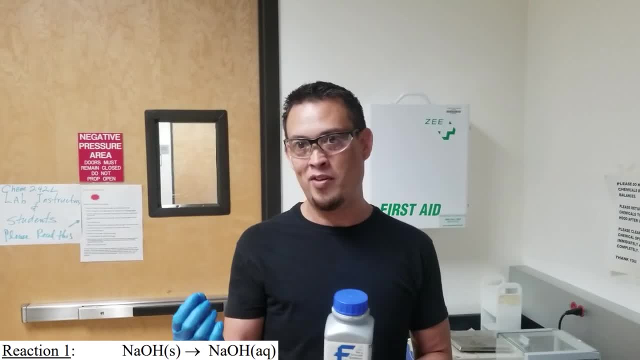 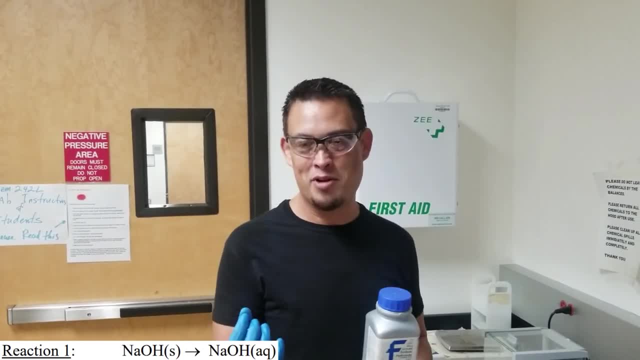 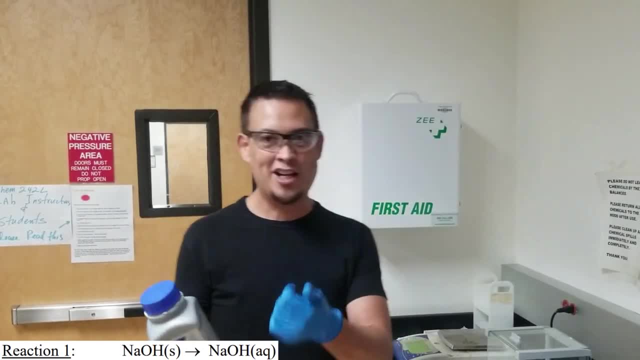 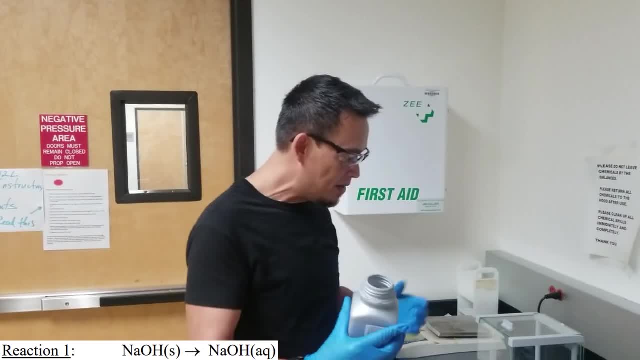 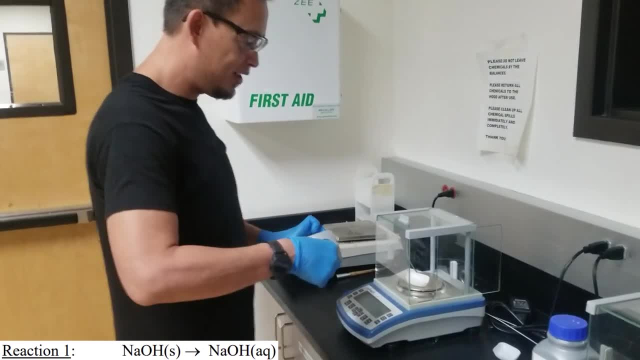 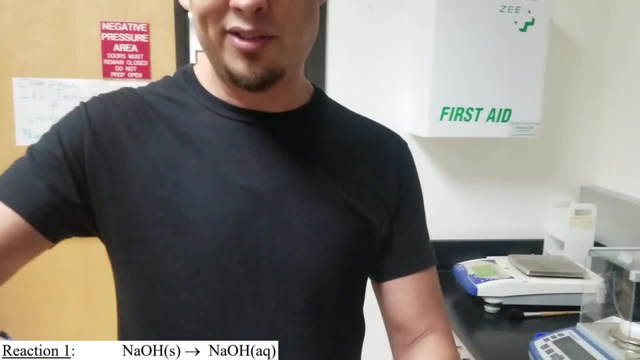 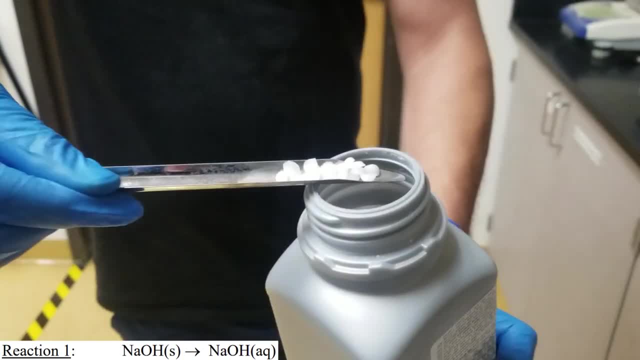 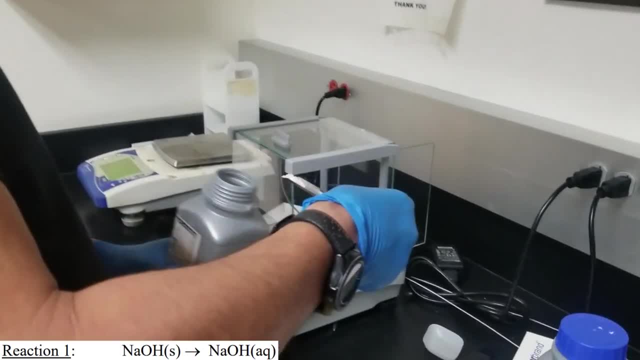 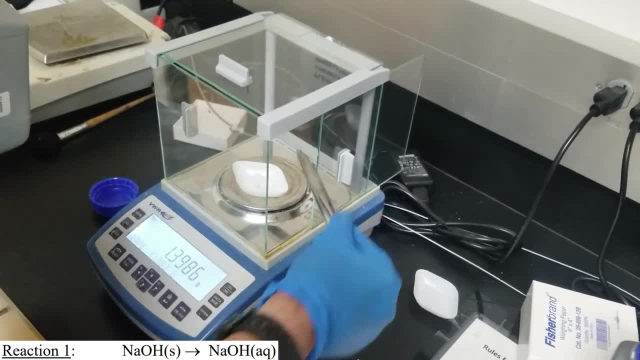 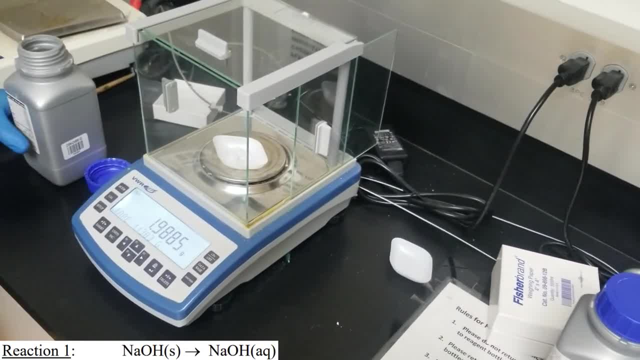 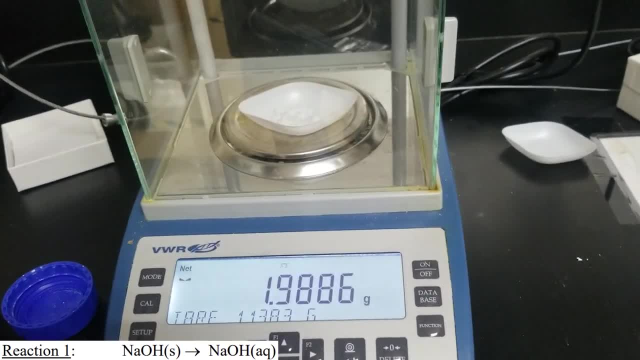 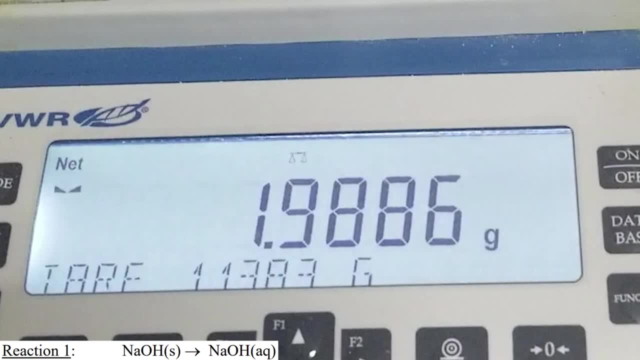 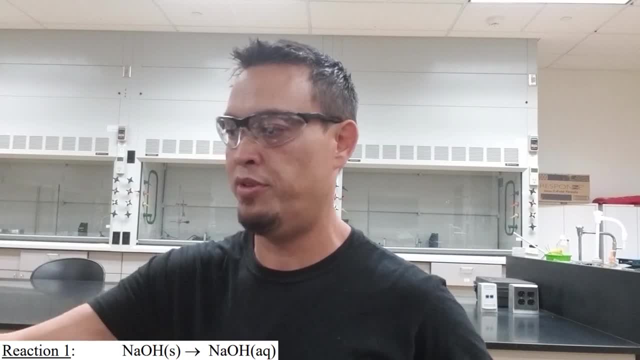 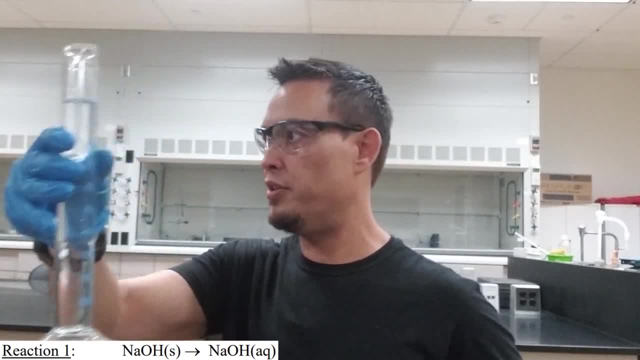 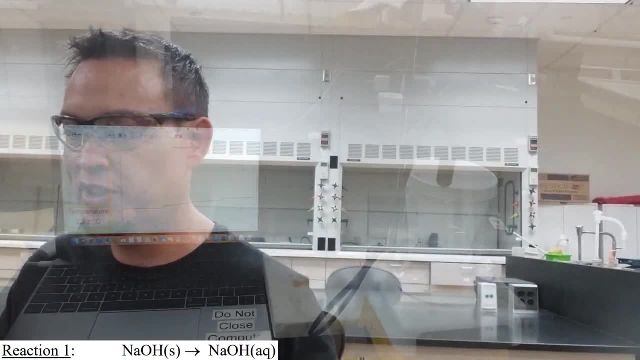 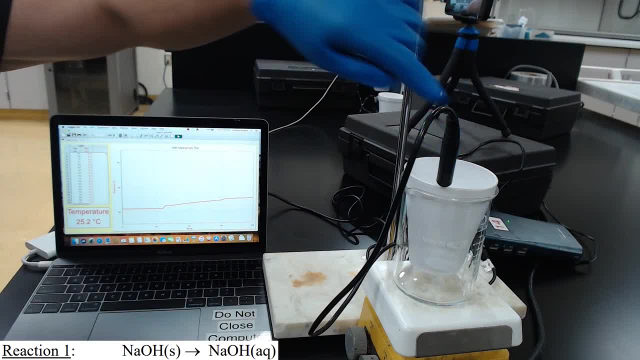 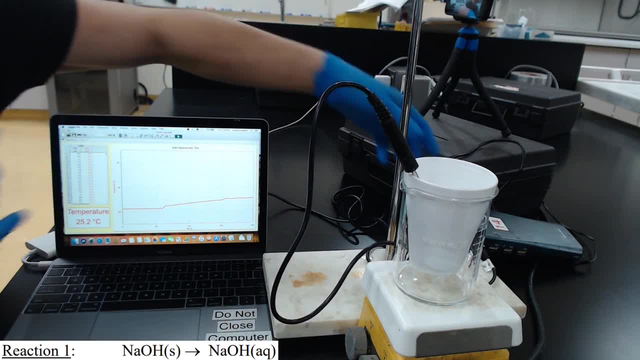 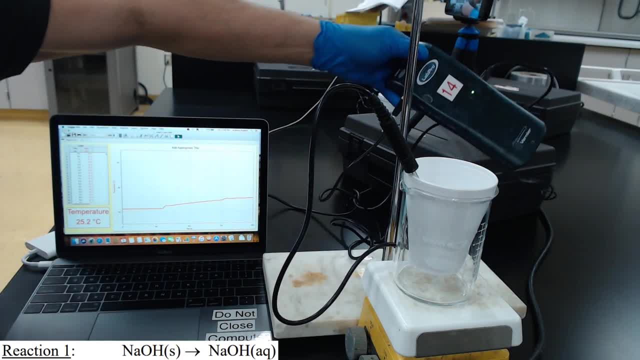 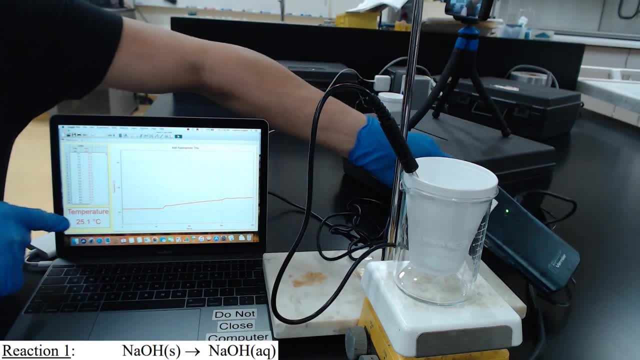 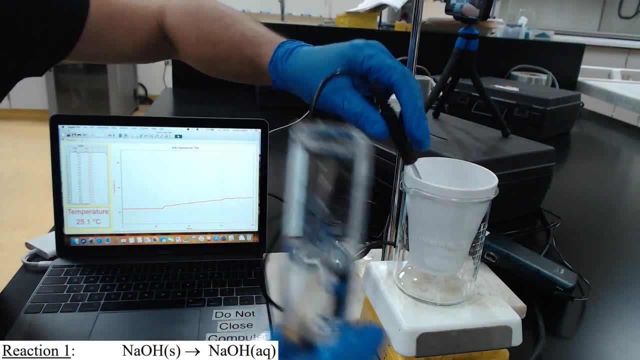 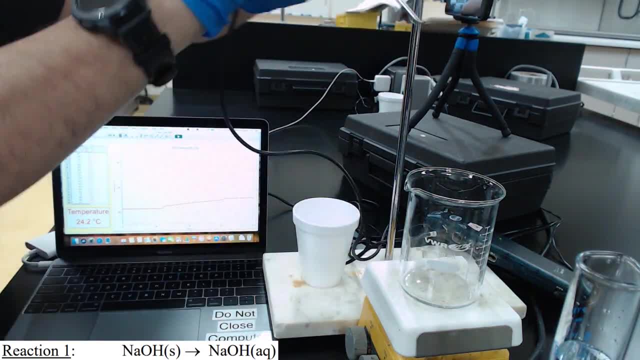 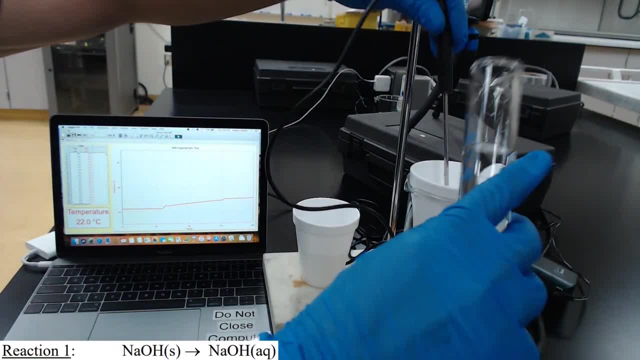 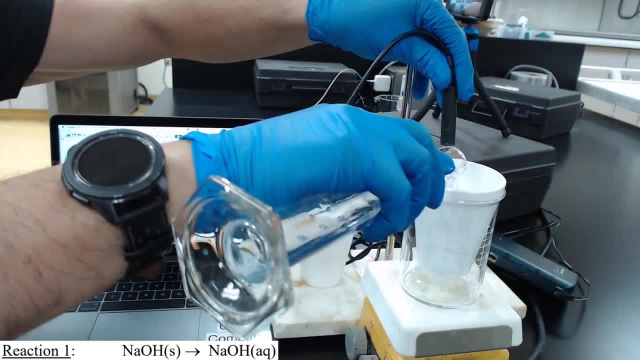 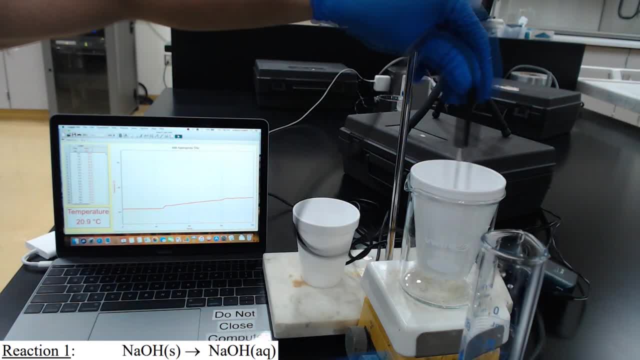 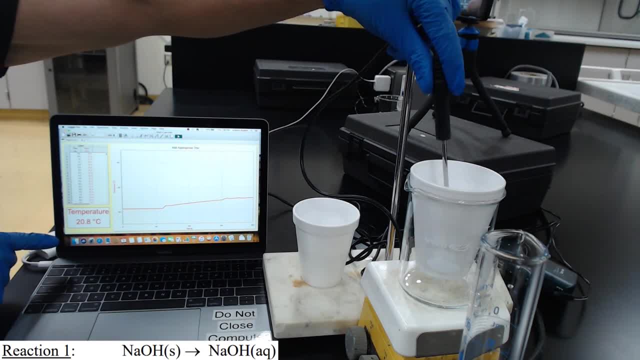 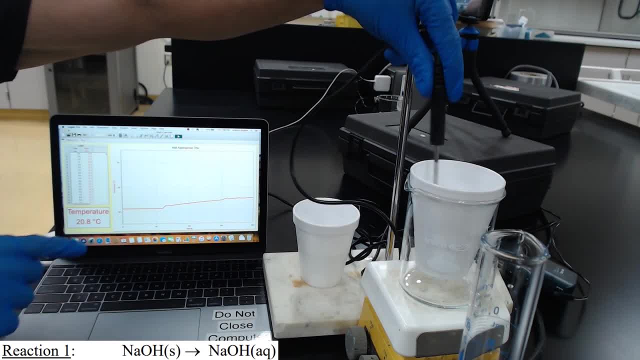 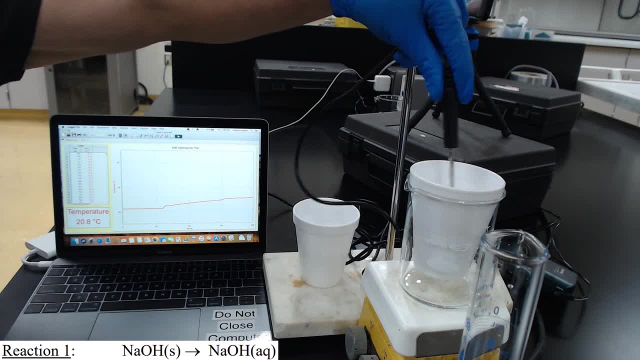 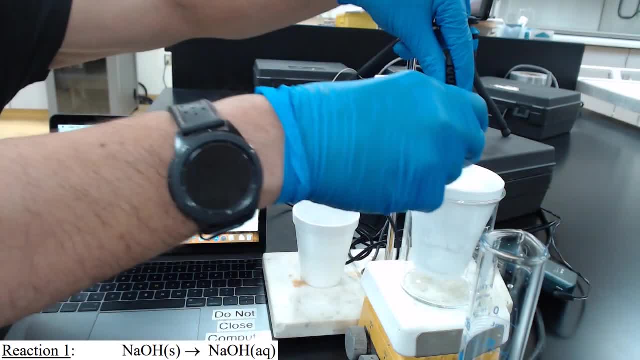 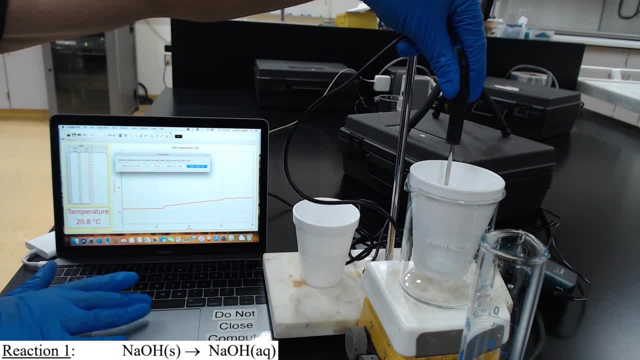 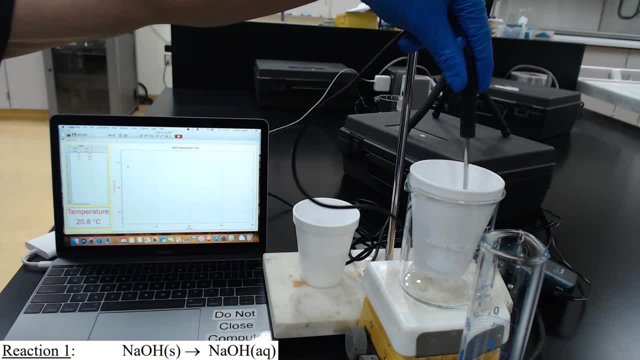 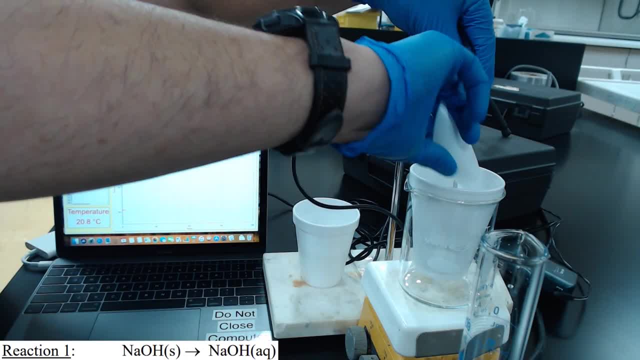 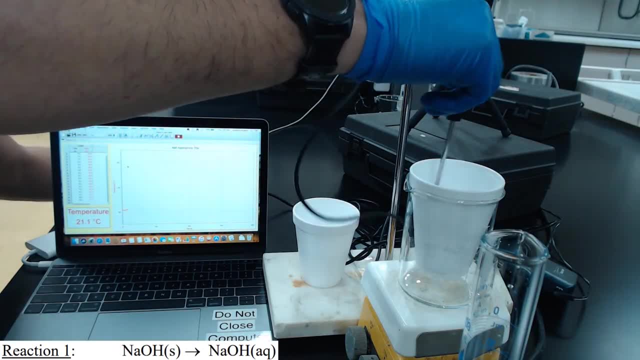 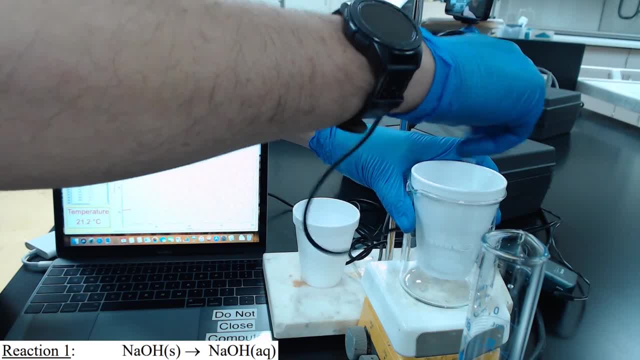 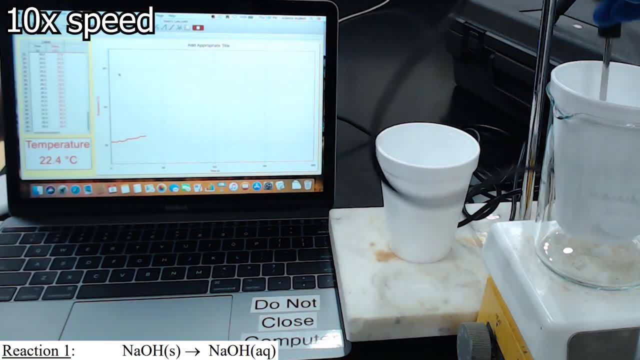 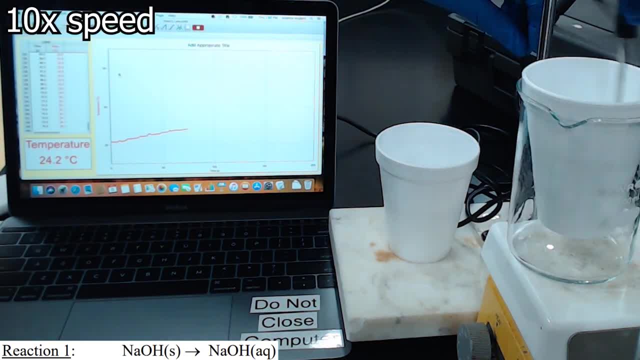 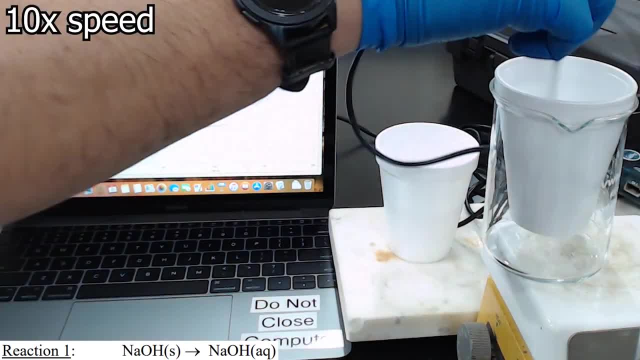 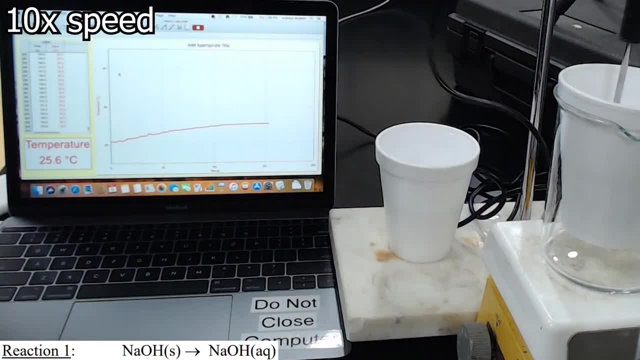 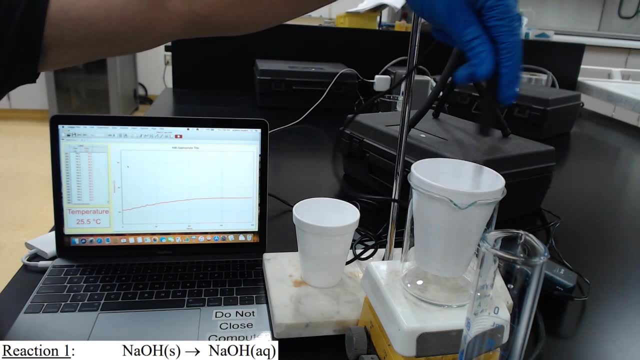 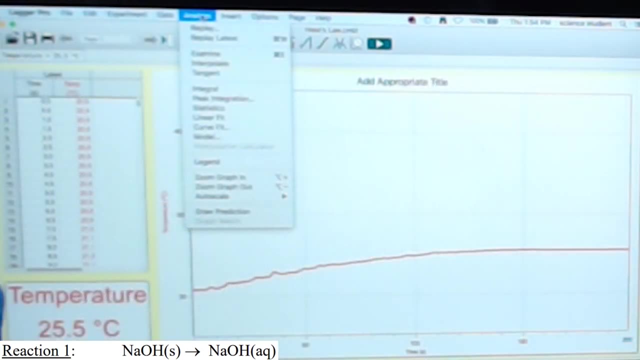 of the sulfur dioxide that we need to make. so, since we have double the quantity of the sulfur dioxide that we need to make so, since we have double the quantity of the sulfur dioxide that we need to make so, since we have double the quantity, Okay. so in order to get the actual data from here, we're going to go to Analyze and Statistics. 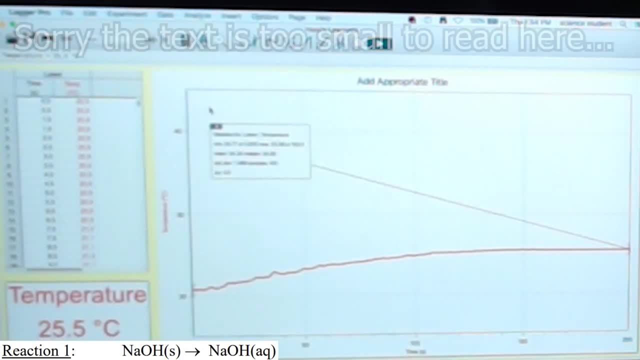 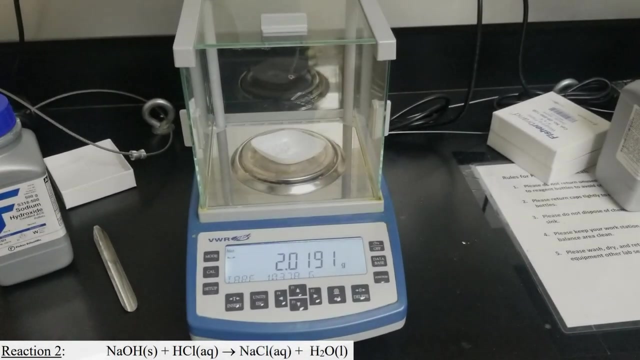 And then we'll look for the min and max here. Okay, so it says the minimum here was 20.77, and our maximum was 25.59.. Okay, I went ahead and weighed out the next sample here, So we have more pellets for the second part of the experiment. 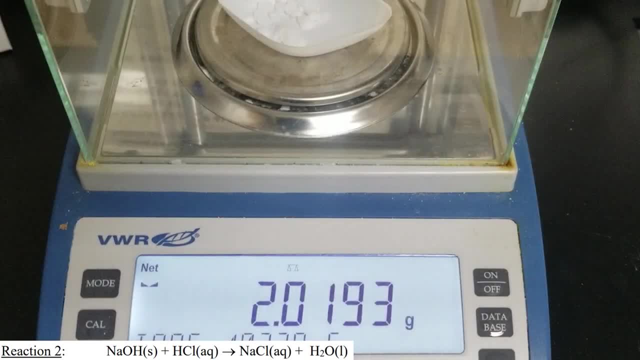 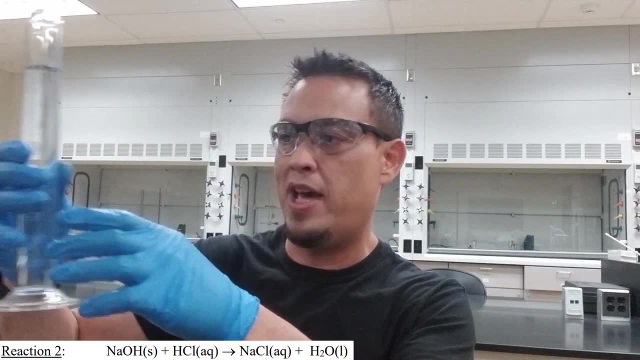 And there is your weight. Make sure you write that down. You're going to need it for the calculations later. Okay, we're all set up now to do the second part of the lab today. Okay, so here I have 150 mils of the 0.5 molar. 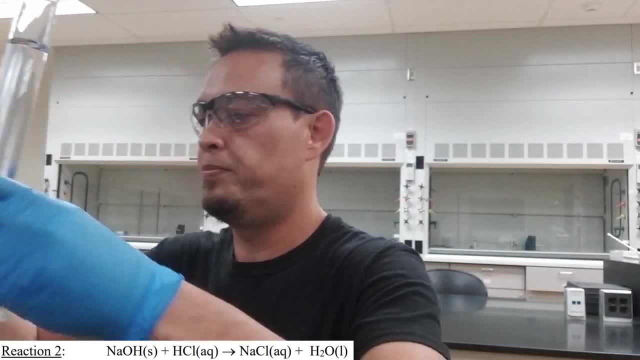 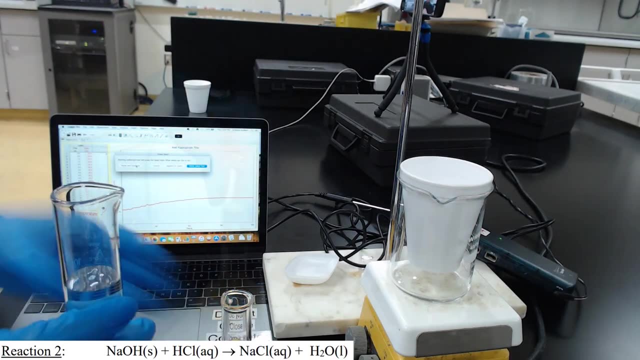 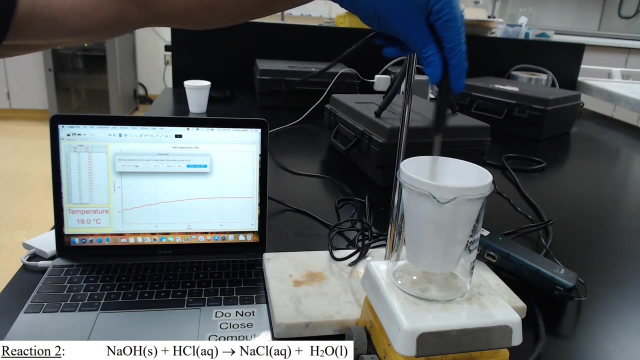 Sorry, 125 mils of the 0.5 molar HCl. So we're going to go ahead and get it in the cup And then I like to make sure the temperature is kind of set before I hit. go on this. 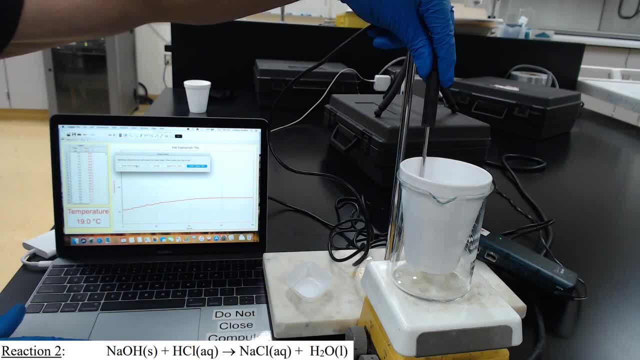 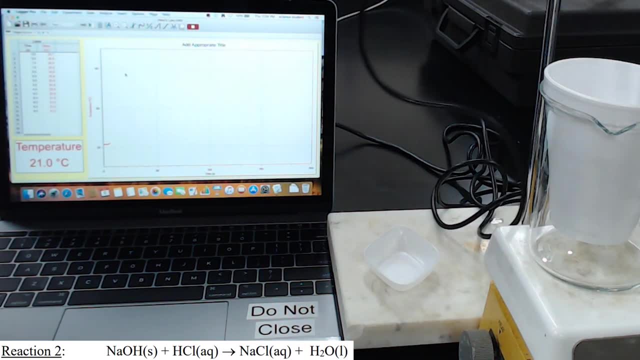 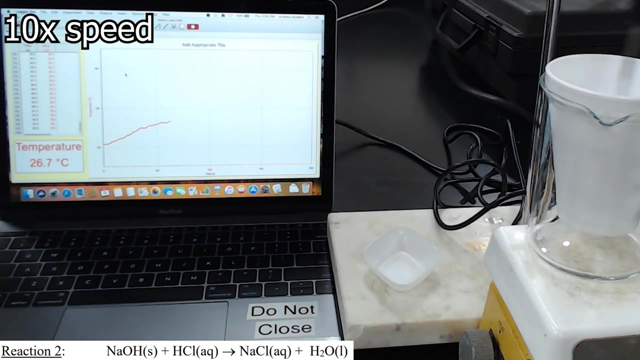 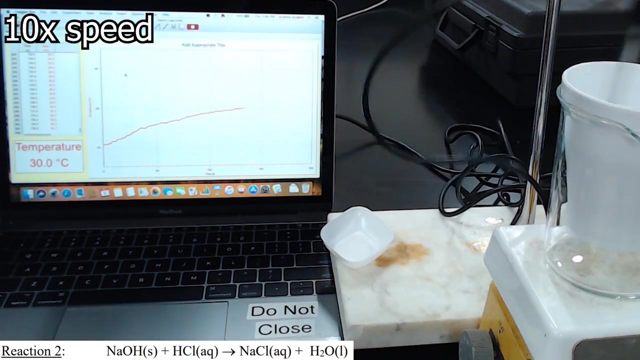 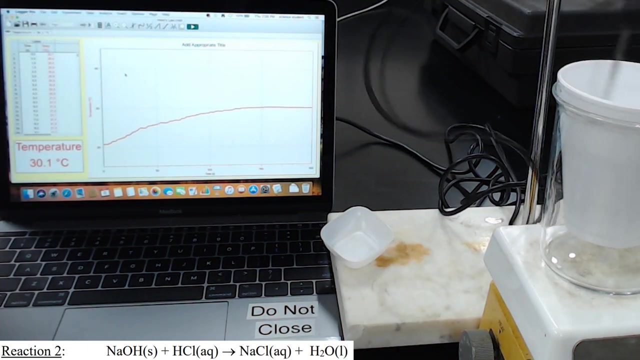 Okay, So we're going to go ahead and start it, and then I'll add the pellets. Okay, so, once again, this is reaction two: solid sodium hydroxide with the aqueous HCl. All right, So this run is done. 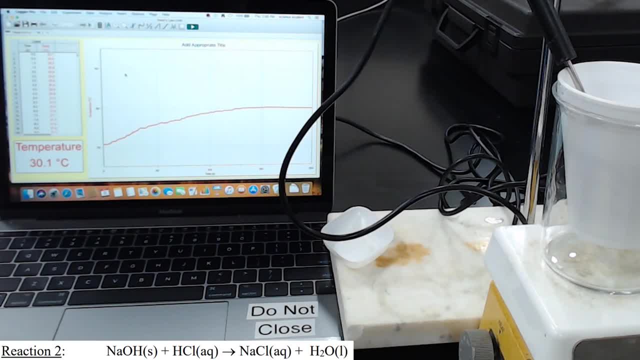 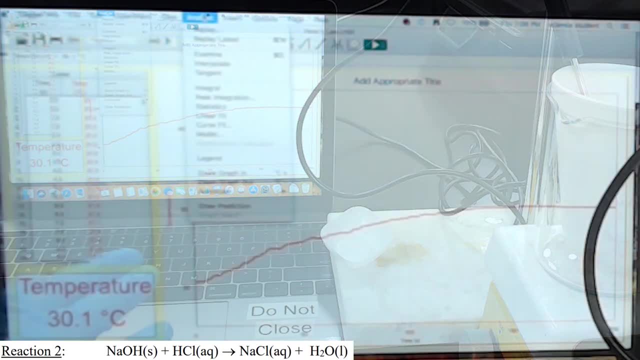 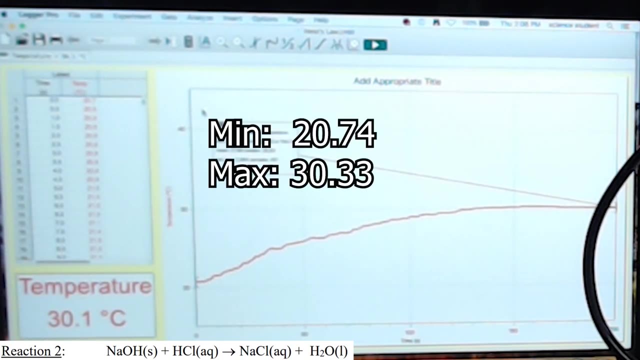 So, just like last time, we were going to analyze the data to get the min and max which you're going to use for your delta T in your calculations. So analyze stats. Okay, So I am seeing the minimum here to be 20.74..